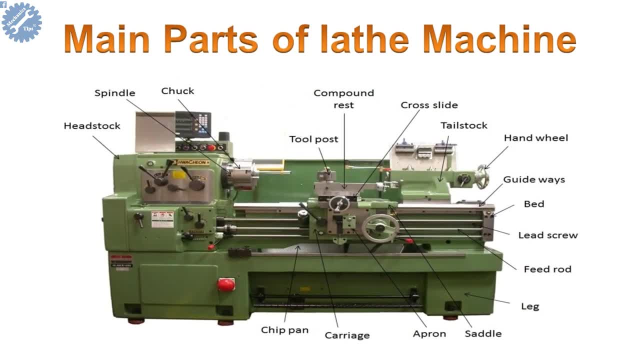 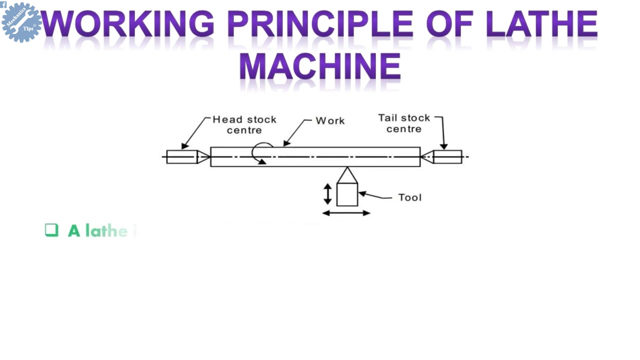 Main Parts of Lathe Machine. Working Principle of Lathe Machine. A lathe is a machine tool which used to removes unwanted materials from a workpiece in the form of chips, with the help of a tool that travels across the workpiece and can be fed deep in work. 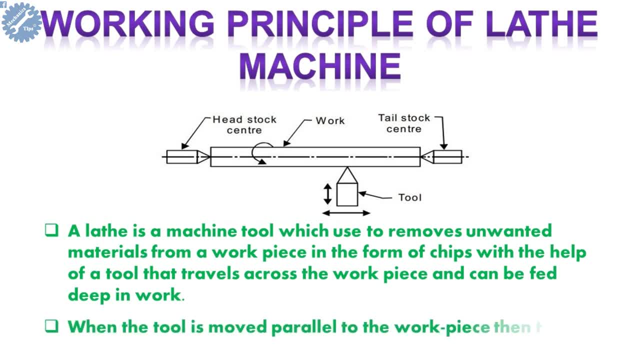 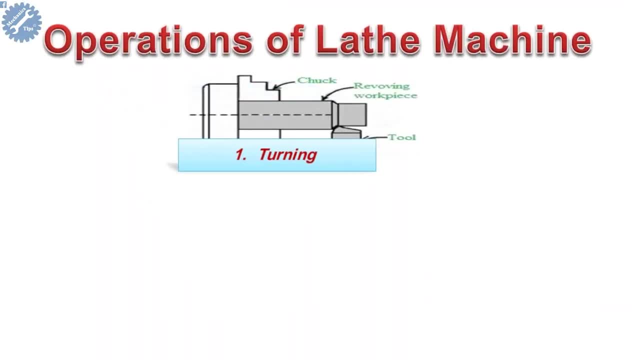 When the tool is moved parallel to the workpiece, then the cylindrical surface is formed. Operations of Lathe Machine. Turning is the operation of reducing the diameter of a workpiece to produce a cover Lathe Machine. The workpiece is either cone shaped or a cylindrical surface, as shown in figure above. 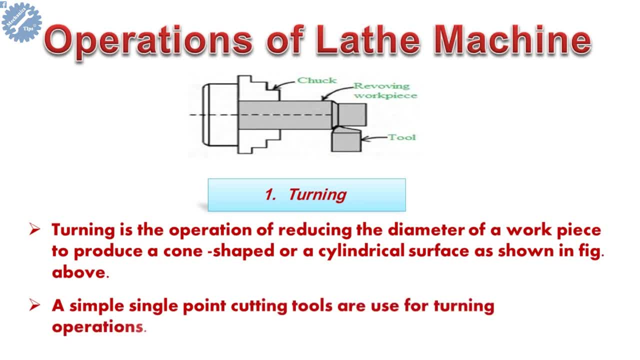 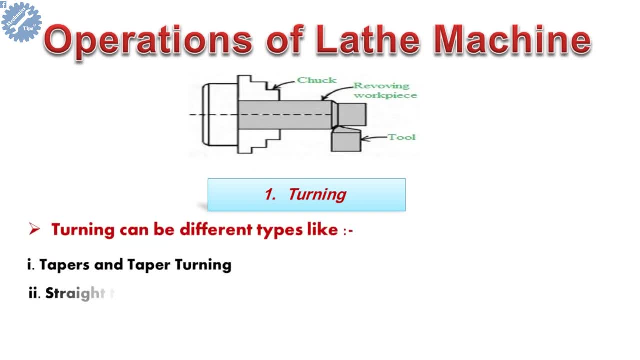 A simple single point cutting tools are used for turning operations. Turning can be different types, like Tapers and Taper Turning, Straight turning, Profiling, External grooving, Facing. Facing is an operation of reducing the length of the workpiece to produce a flat surface, square with the axis. 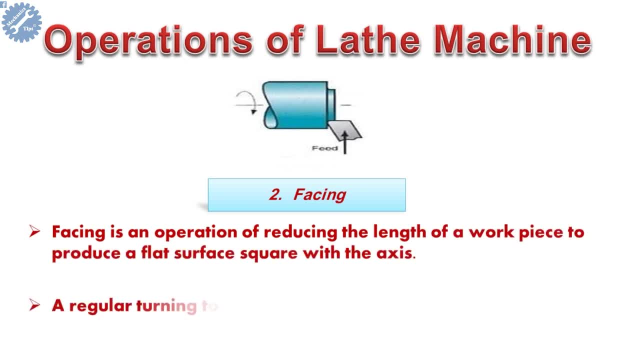 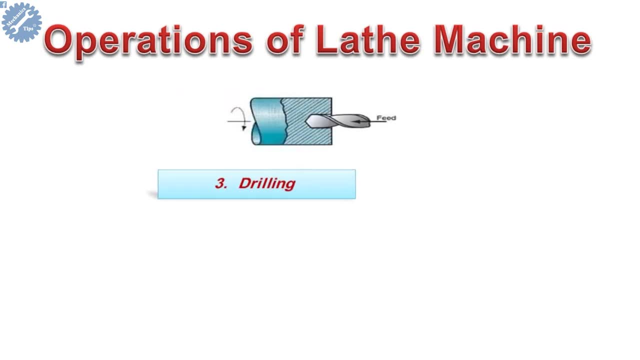 flat surface square with the axis. A regular turning tool may also be using for facing a large workpiece. Drilling is an operation of producing a cylindrical hole in a workpiece by the rotating cutting edge of a cutter known as the drill. Boring is the operation of enlarge a hole or cylindrical cavity to produce circular 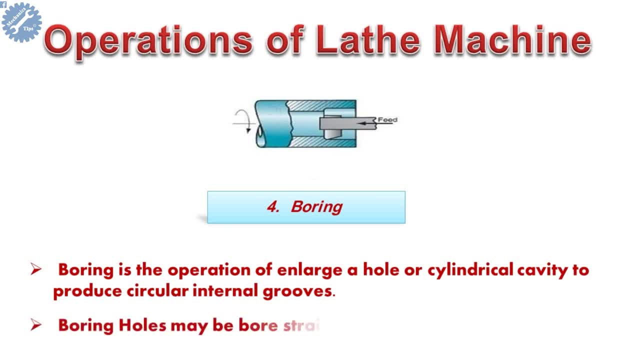 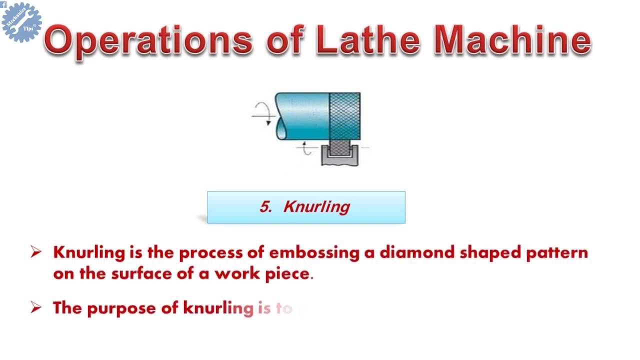 internal grooves. Boring holes may be bore straight and tapered. Knurling is the process of embossing a diamond shaped pattern on the surface of the workpiece. The purpose of knurling is to provide an effective gripping surface on a workpiece to prevent 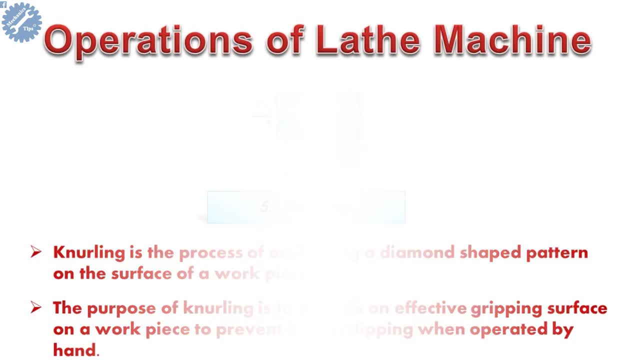 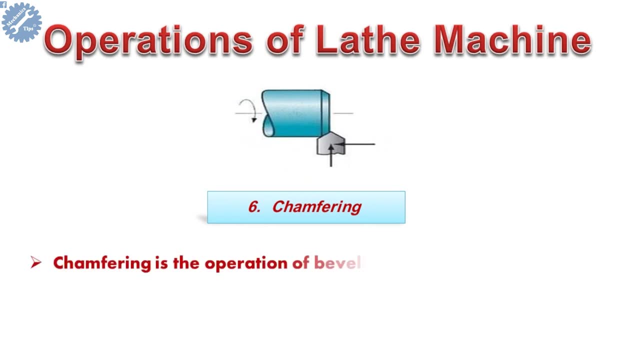 it from slipping when operated by hand. Parting is the operation of beveling the extreme end of a workpiece. This is done to remove the burrs, to protect the end of the workpiece from being damaged and to have a better look.